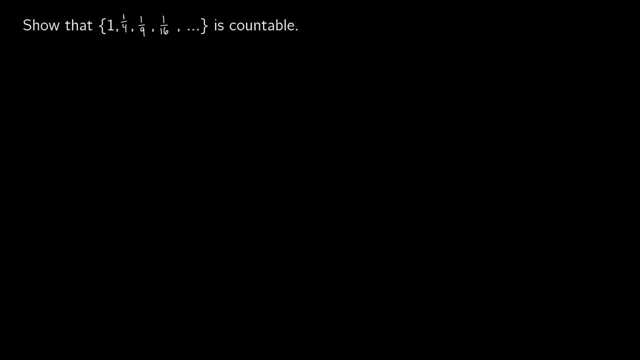 We want to show that 1,, 1 4th, 1 9th, 1 16th is countable. So what we want to do is take this original set and then map it on to the natural number 0,, 1,, 2,, 3, and so on. We don't necessarily. 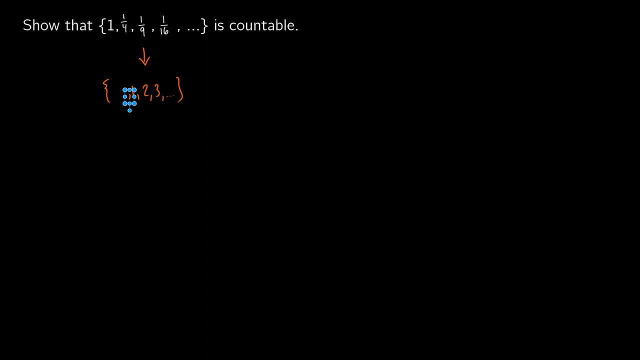 need to include 0 in this one. we're just removing one number. So for the sake of simplicity, I'm going to remove 0 here. that way we have a nice formula. What we notice about our original set in this case is that this is of the form 1 over 1 squared. I'll just put the numbers in there. 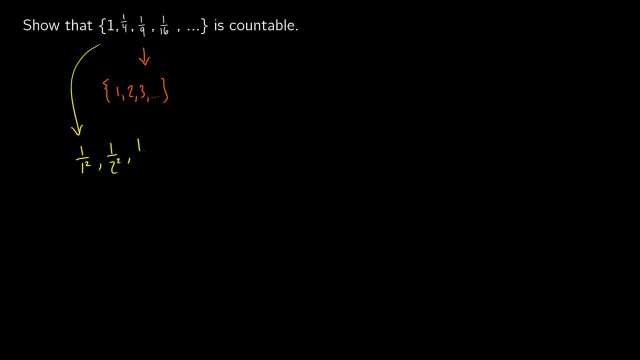 1 over 2 squared, 1 over 3 squared, and so on. So, in other words, we'd be taking any of our forms- 1 over n squared- and trying to get them matched up with n. So what we can do? 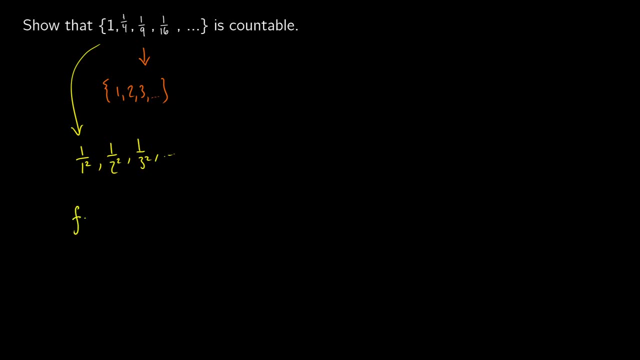 is, we can take a function and we can say, okay, this function is going to go from the natural numbers to our set: 1, 1, 4th and so on. So we'll take a number from our natural numbers and we're going to just simply map it on to 1 over n squared. So f of n is equal to 1. 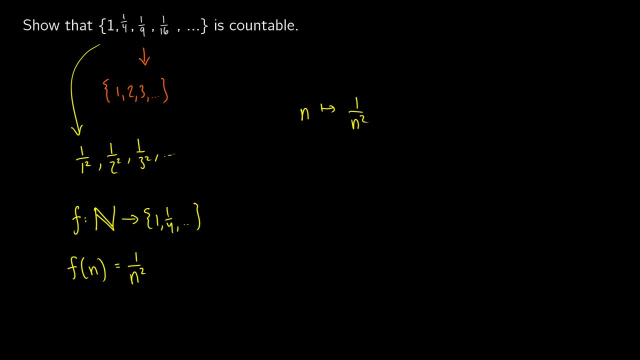 over n squared, And because we get a nice mapping from our set to the natural numbers and by doing that we're going to be able to get a number from our set to the natural numbers And vice versa, because it's a bijection, we can claim that this is therefore countable. 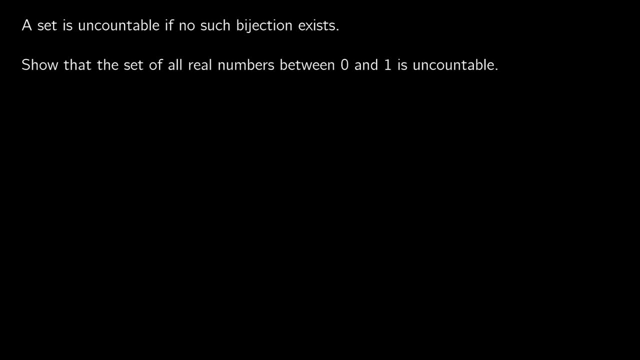 So what happens if you want to show that something is uncountable? That means that no such bijection exists. So for this exercise, we're going to show that the set of all real numbers between 0 and 1 is uncountable. So what we're going to do is we're going to assume that it's countable. 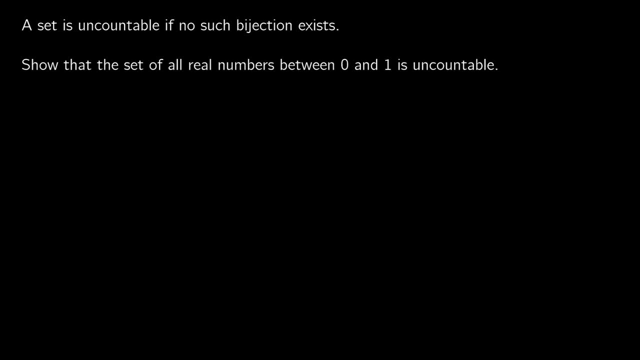 and all of the numbers are countable. So we're going to show that the set of all real numbers between 0 and 1 exist. So, in other words, we're going to get like 0.0001, 0.02456.. Basically, 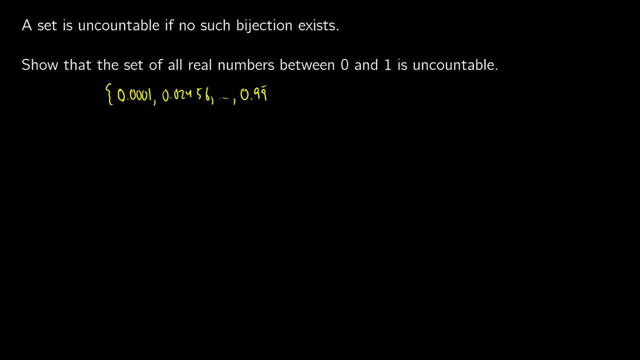 we're just going to get all of the numbers up until, like, let's say, 0.99 repeated. I know that's equal to 1, but for the sake of showing it, let's just assume it's not Okay. so for this one, we're going to be clever. What we're going to do is we're going to take our set. 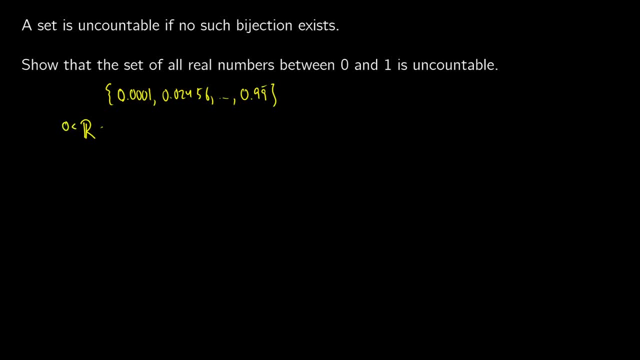 of all of these real numbers. So let's call this the set R between 0 and 1. We're going to order these, So we're going to say the first number is A1, the second one's A2, third one's A3. And that just continues on until we get to say AN, which would be our. 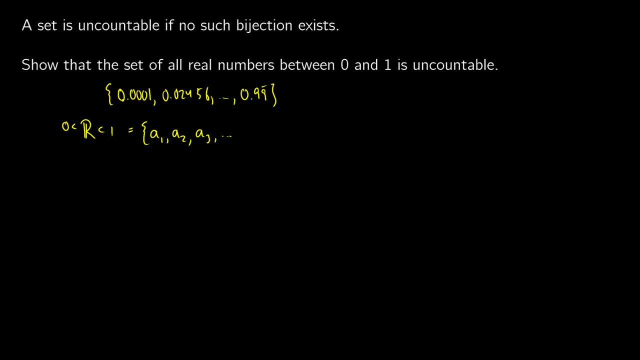 maybe not our last number. So let's just say that's our set of all real numbers. Let's just leave it like this, going on from A3.. And what we're going to do is we're going to write these numbers out. So let's say, for the sake of example, that A is 0.7362, and some more. 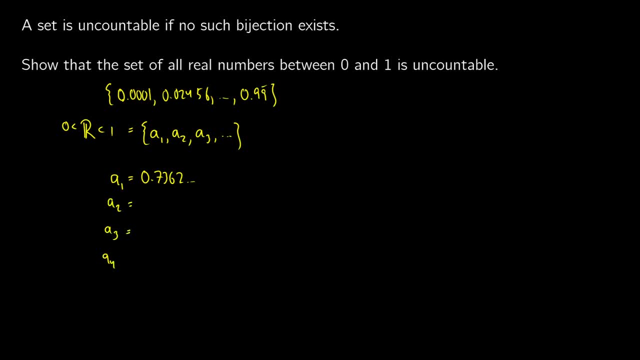 A2,, A3, and A4 is going to be, let's say, 0.1295 keeps going, 0.6311 keeps going and 0.525.. 0.5124 keeps going. Okay, So if our set is countable, all of our numbers should be. 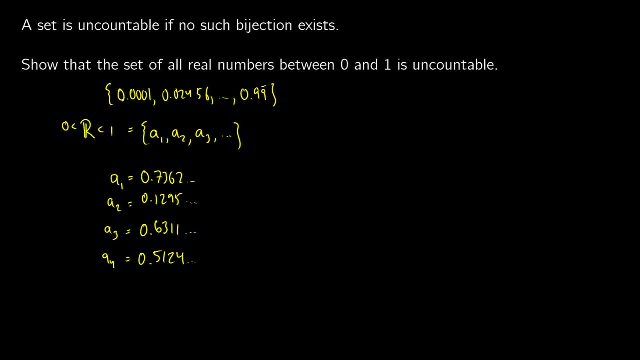 accounted for. But what we're going to show is that we can make a new number. that wasn't in our original set. Because we can make a new number, we'll show that it is uncountable. So what we'll do is we're going to pick our new number. we're going to call it R. 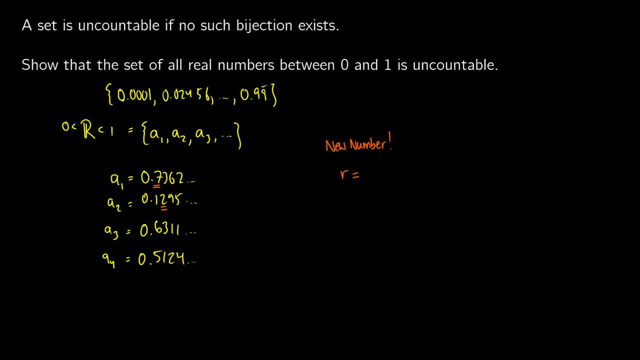 and how we're going to do that is, we're going to call it R and we're going to call it R, and what we're going to do this is we're going to change the number in one position in each of our A1s. So, in other words, let's say that R is 0.. 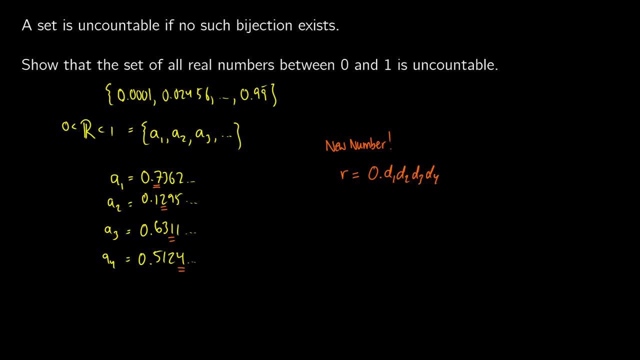 Say D1, D2, D3, D4, and so on, And what these are in this place are just our decimal points. So D1 is the 10th place, D2 is the 100th place, and so on. 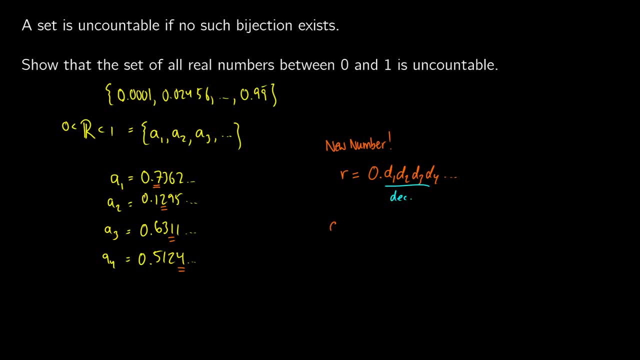 And how we're going to define this is we're going to say that D- I. so the ith position is going to be one of two things: It's going to be 2 if A- I- I is not equal to 2.. 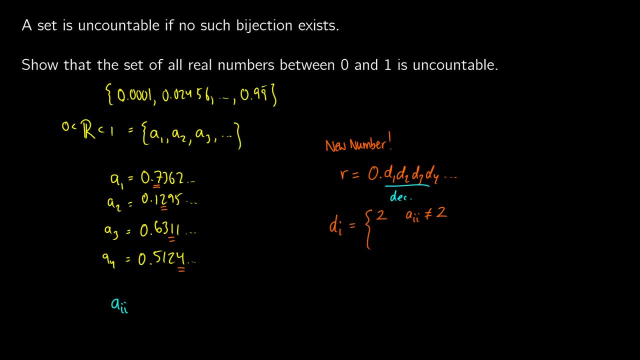 So let me explain this: If we have A I I, then what this means is that A11 would be the first decimal. If we have A22, that would be second number and that would be second decimal. So in other words, we're basically going to change the first bit in A1 to be 0.2 if we don't have a 2 in that 10th place. 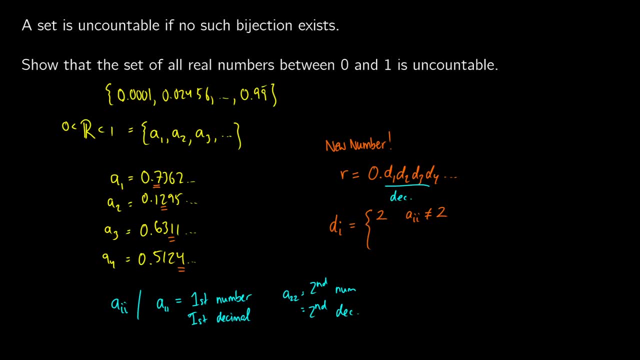 And we're going to change it to. I'll try to revert back to the previous color, the 3. if A, I, I is equal to 2.. So, in other words, if the third position of the third number is 2, we'll turn it into 3.. 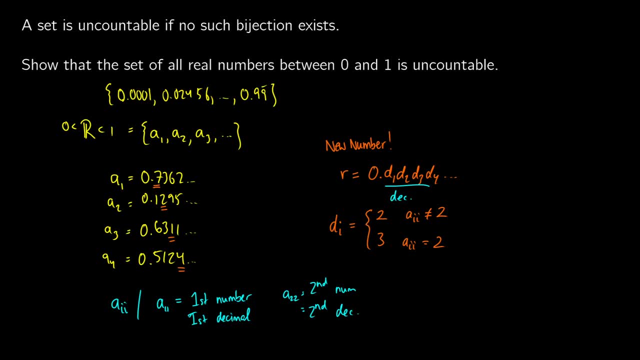 Now what we're going to get in this case is a brand new number We're going to get: R is equal to 0, and in this case, because the first place is 7, we change it to 2.. In the second position, it's 2.. 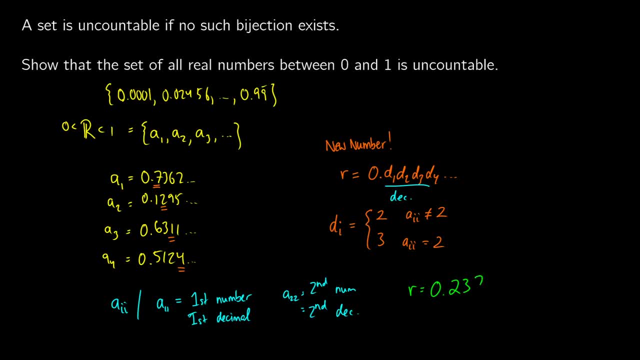 So we change it to 3.. In A3, it'd be 1.. So we change it to 2.. In A4, it would be 4.. So we change it to 2.. And this continues on, and on, and on. 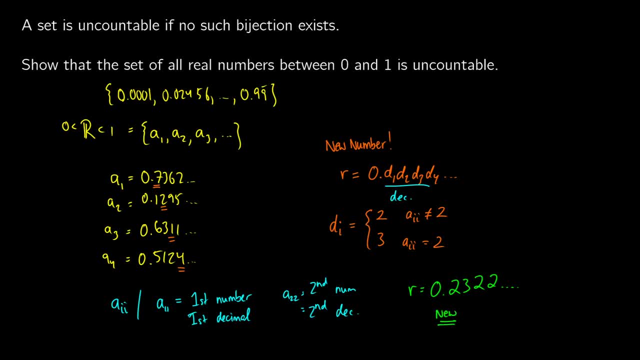 Now this has to be new, because we're going through every single element and we're changing it. So you might say we already have that number in our set because we're accounting for everything, But then let's say that R or something very similar to R would be in our set. 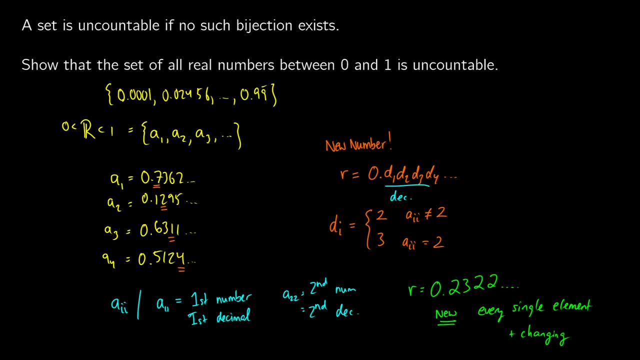 As soon as we get to whatever position R is in our original set, we are going to change one of those values. So, because we can create this new number that hasn't been mapped to the natural numbers in the first place, we can then claim that this set is uncountable.